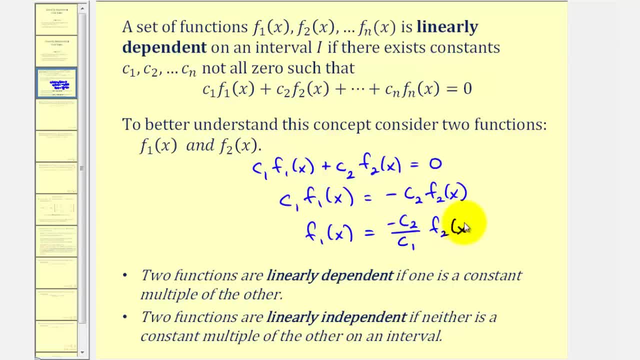 which is just another constant times f sub two of x. So we can say that two functions are linear dependent if one is a constant multiple of the other. In this case the constant would be negative: c sub two of c sub two divided by c sub one. 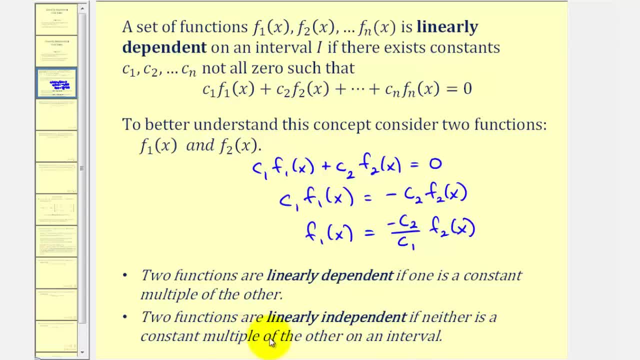 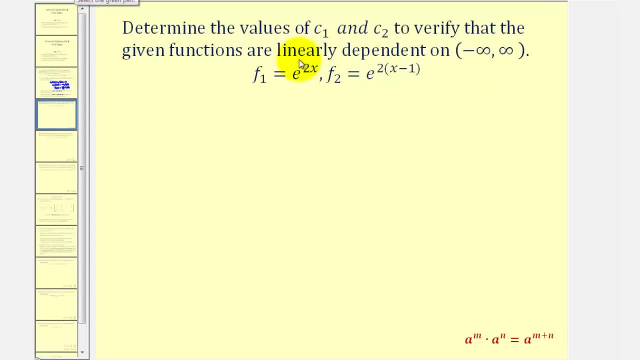 Two functions are linear independent if neither is a constant multiple of the other on a given interval. Let's take a look at our first example. We want to determine the values of c sub one and c sub two to verify the given functions are linear dependent. 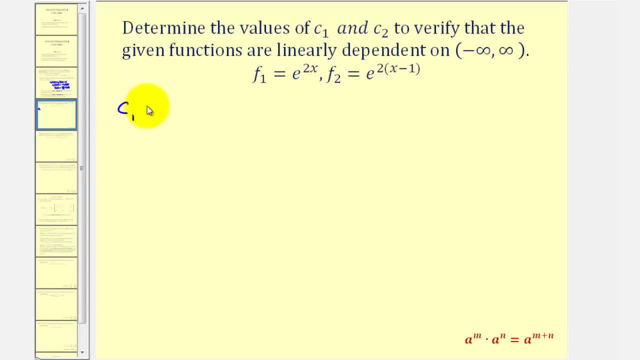 which means c sub one, some constant times, e to the power of two, x plus c sub two times e raised to the power of two times the quantity x minus one must equal zero. Let's start by distributing here, which would give us c sub one, e to the two x. 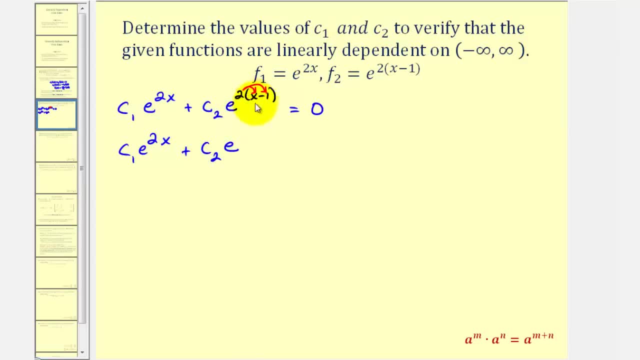 plus c sub two e to the power of this would be two x minus two, which I'm going to write as two x plus negative two. just to emphasize that we can now apply this property of exponents here, meaning because we have a sum here. 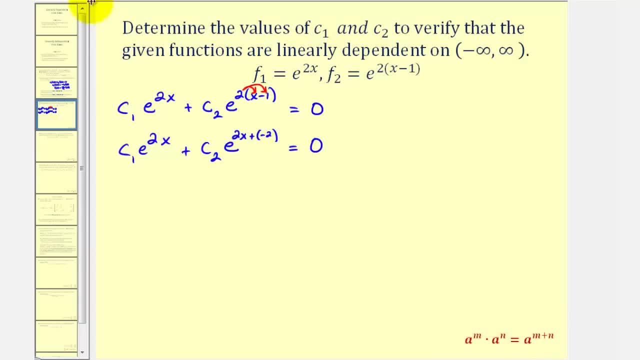 we can make this as a product with the same base. We can write this as: c sub one, e to the two x plus c sub two, e to the two x times e to the power of negative two equals zero. Well, e to the negative two is just another constant. 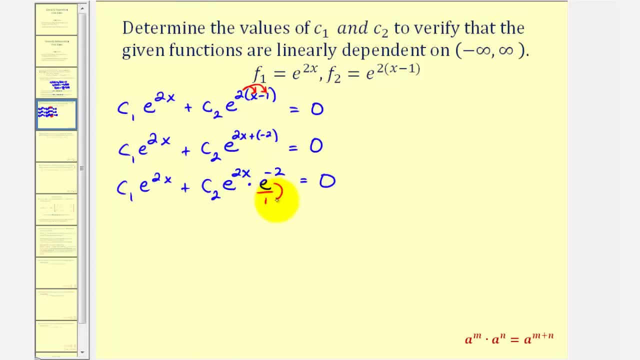 and we can write this using a positive exponent if we move it down to the denominator. Now, let's write this as c sub one, e to the two, x, e to the two, x plus. since c sub two is also a constant, let's write this as c sub two divided by e, squared. 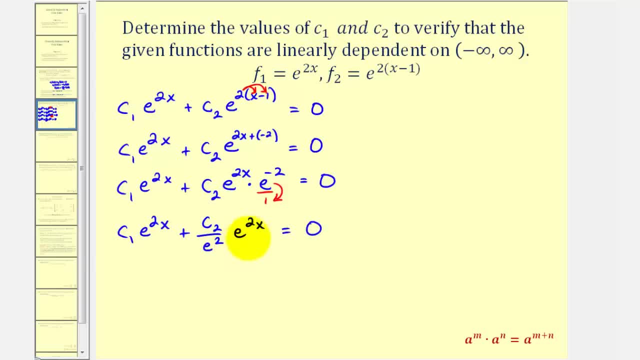 e to the two x equals zero. Now, if we take a look at the exponential parts, notice how they're both e raised to the power of two x And therefore, if these are opposites, this sum would be zero. So let's go ahead and let c sub two be equal to e squared. 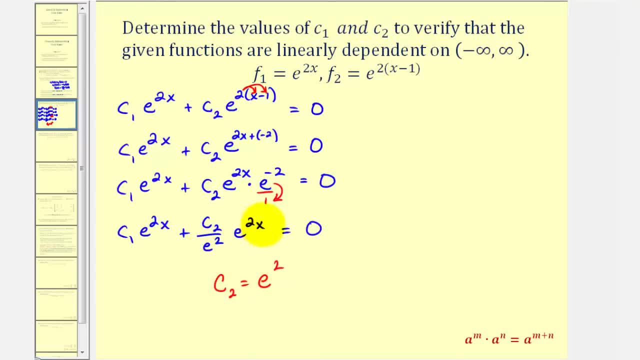 which would make this positive one e to the two x. And therefore, if we let c sub one be equal to negative one, this would be negative e to the power of two x. So just to verify, if c sub one is negative one, 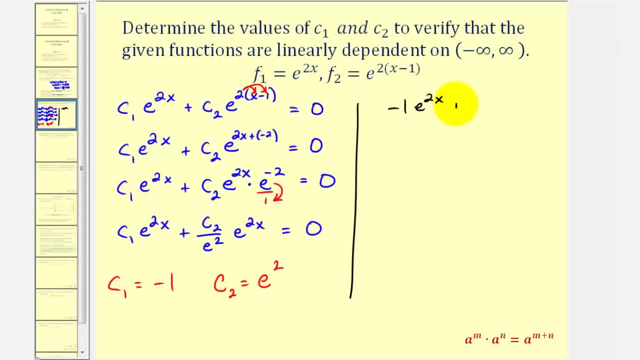 we have negative one e to the power of two x plus c sub two is e squared. Notice how here we'd have negative e to the two x and here we'd have plus e to the two x, which is equal to zero, And therefore we verify the given functions. 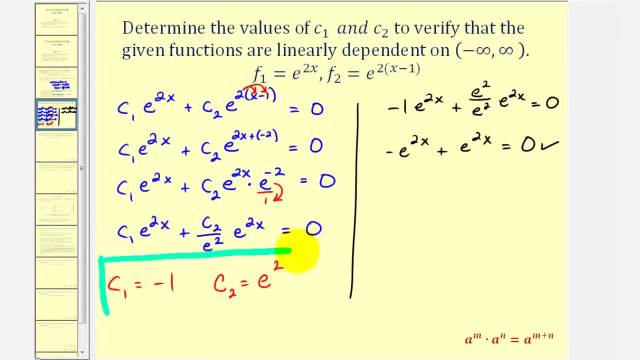 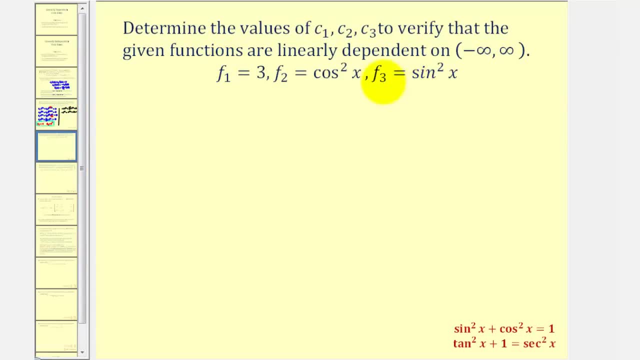 are linear dependent, with this value of c sub one and this value of c sub two. Let's take a look at another example. Again, we want to verify. these three functions are linear dependent but determining the values of c sub two. So c sub one, c sub two and c sub three. 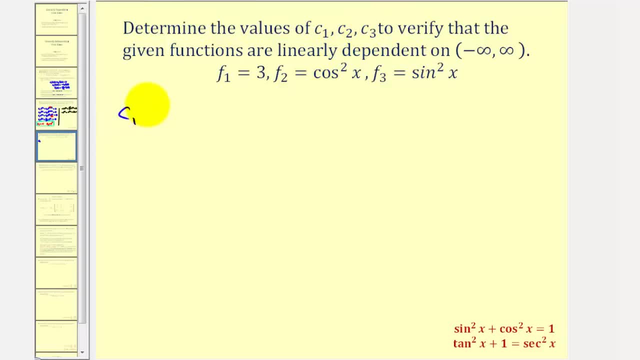 they would satisfy the given equation: C sub one times three plus c sub two times cosine squared x plus c sub three times sine squared x equals zero. Well, having this cosine squared x and sine squared x here should remind us of this identity here. 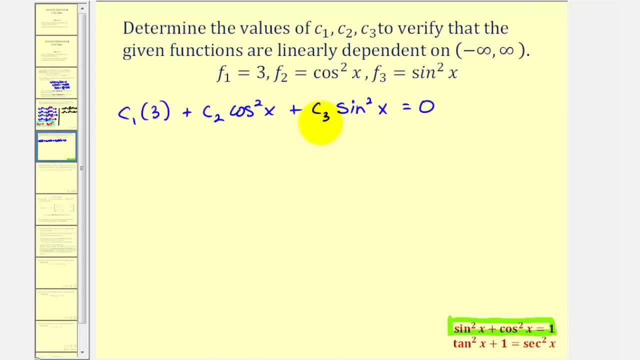 So if we let c sub two be equal to one and c sub three be equal to one, this sum here would be equal to positive one. So if we can make this product here negative one, we can verify. these are linear dependent functions. 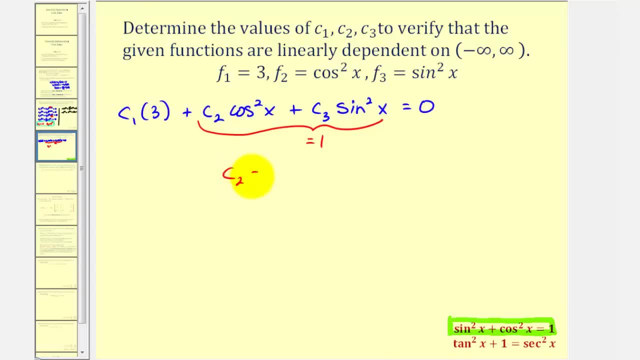 So again, this equals one. if c sub two equals one and c sub three equals one, Well, three is the same as three over one. so we multiply it by the reciprocal or 1 third. So this would be positive one. 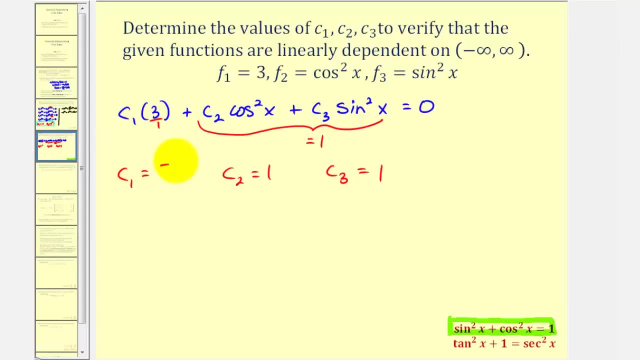 And since we want negative one, we'll let c sub one be equal to negative 1. third. Again, let's go ahead and verify. We'd have negative 1 third times three plus again c sub two and c sub three are equal to one. 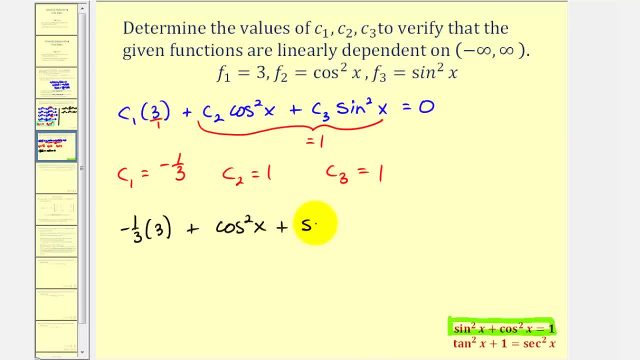 So we just have cosine squared x plus sine squared x equals zero. Well, this product here is negative one and this sum here is equal to positive one, verifying that we do have three linear dependent functions verified by these three values of c. Let's take a look at one more example. 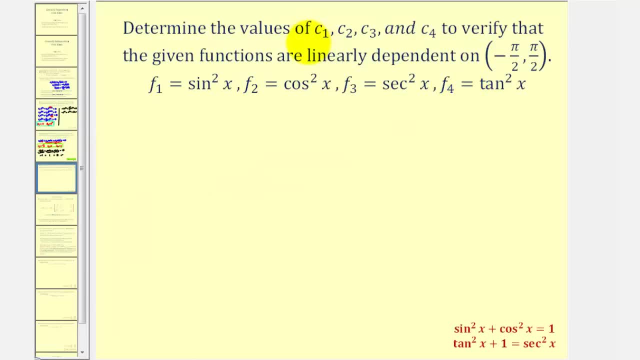 where here we have four different functions. so we'll have to find c sub one through c sub four. So we'd have c sub one times sine squared x plus c sub two times plus c sub three times c squared x plus c sub four times tangent squared x. 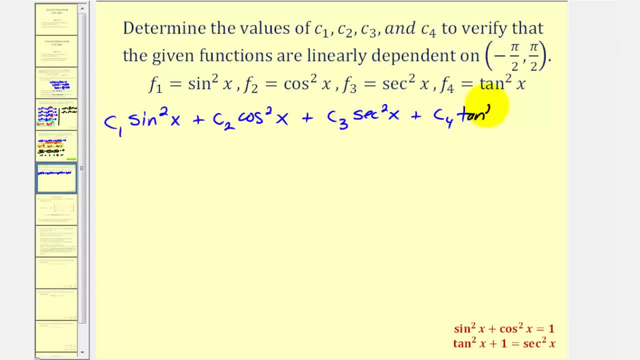 must equal zero for some values of c if these are linear dependent functions. Well, from our last example we should be able to recognize that if we let c sub one be equal to one and c sub two be equal to one, this sum here would be equal to positive one. 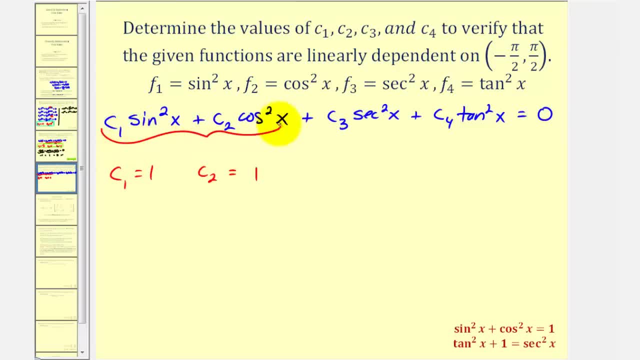 So now, if we get this sum here, we should be able to recognize that if we let c sub one be equal to one. so now, if we can determine the value of c sub three and c sub four, that would make this sum equal to negative one. 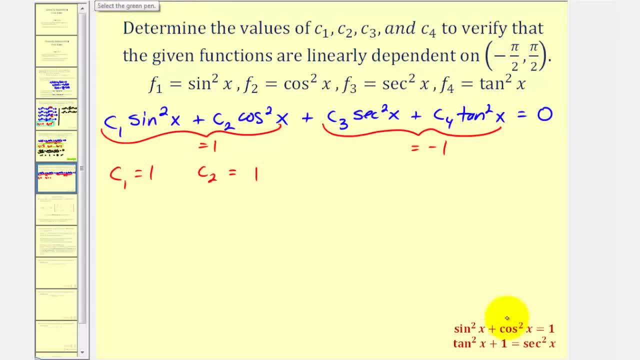 we would satisfy the equation. So, looking at the identity here, tan squared x plus one equals secant squared x. notice, if we subtracted one on both sides and subtracted secant squared on both sides, we would have tangent squared x minus. secant squared x equals negative one. 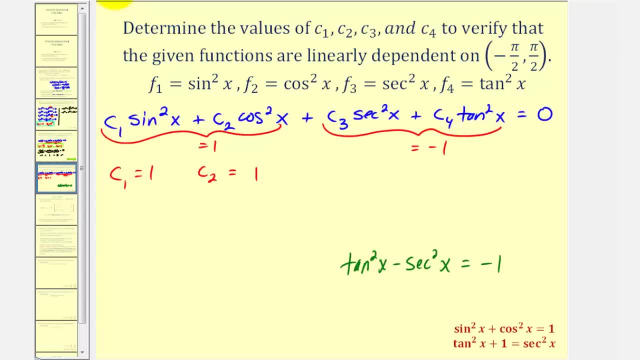 which means if we let c sub four be equal to positive one and c sub three be equal to negative one, to get the minus secant squared x, we would satisfy the equation. So again, let's go ahead and verify this: C sub one and c sub two are one. 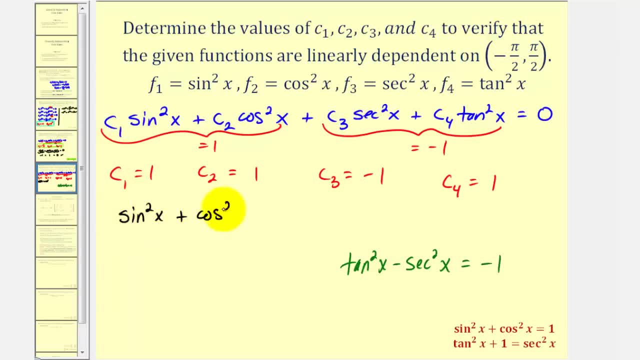 We have sine squared x plus cosine squared x, and then c sub three is equal to negative one. so we have minus secant squared x, c sub four is one, so plus tangent squared x equals zero. Well, this sum is one.